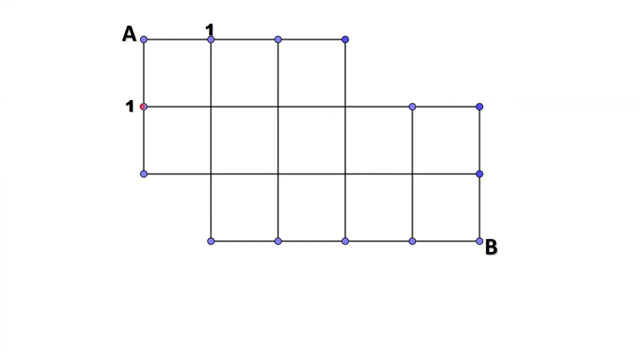 You only have one way, because you cannot go back. You cannot go to the left like this. It's impossible. Move to the next stage. To reach this point, you have different ways. You can reach this point from this point. Also, you can reach this point from: 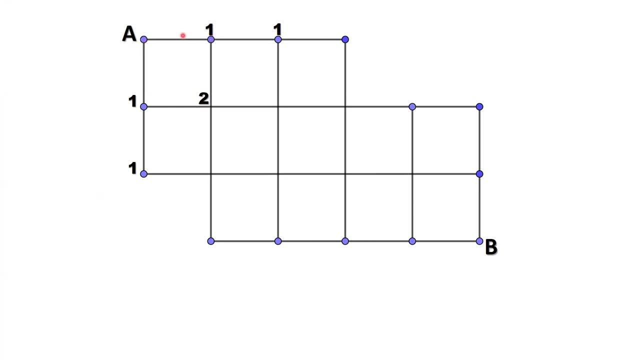 the top point. To reach this point. you have one way To reach this point. you have one way To reach this point. you have one plus one, two different ways. So here the number should be two. Now consider this number. Why this number is one? 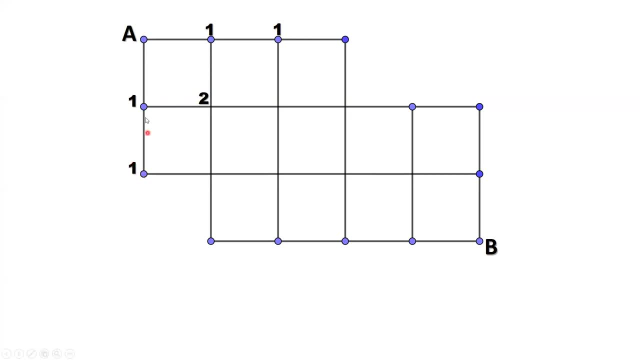 Because you can only move down from this point On the left-hand side. you don't have a point, So this point only can be reached from the top point. You only have one way. Similar discussion for this point. This point only can be reached from the point on the left. 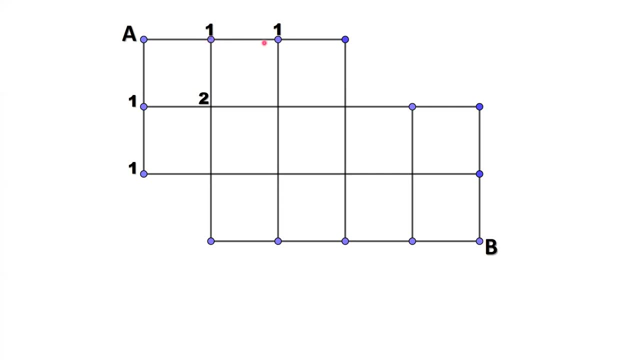 To reach this point you only have one way. So here you only have one way. Let's move on. Look at this point. This point can be reached from the top point or the point on the left. Here is two, Here is one. One plus two equals three. 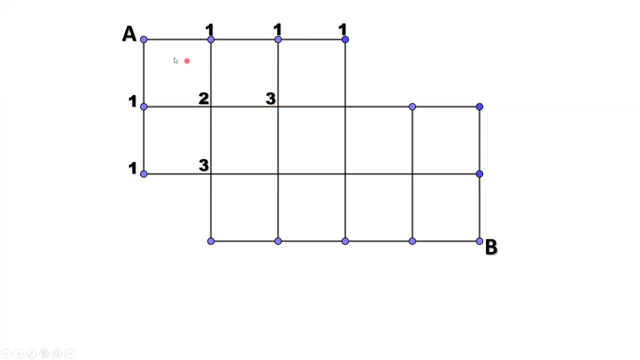 You have three different ways to reach this point from point A. Similarly, for this point you have one way from the point on the left, Two ways from the point on the top. One plus two equals three. From A to reach this point totally, we have three different ways. 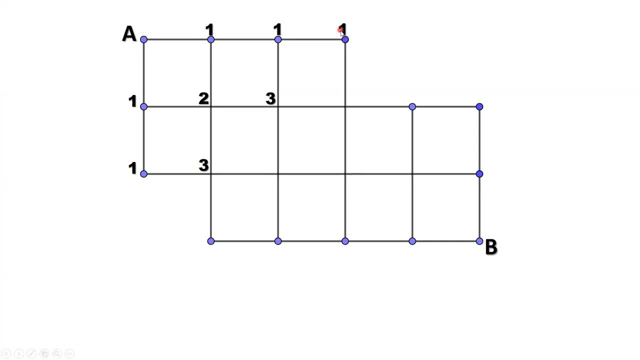 Similarly for this point. you don't have a top point, You only have a point on the left. So one plus zero equals one. Follow the sequence: One plus zero equals one. One plus zero equals one. One plus zero equals one.